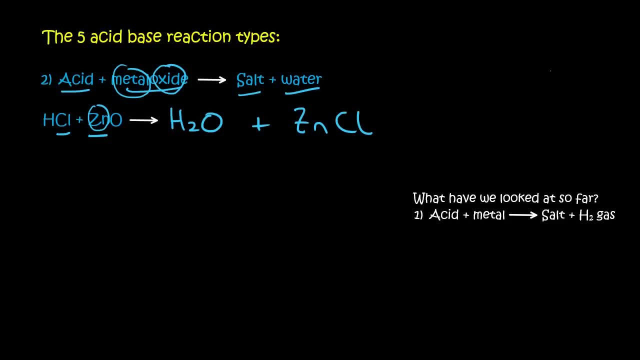 And so that's the salt, Always the metal first, then the non-metal. Now we saw that chlorine has a valency of minus one, zinc is positive two, and so that means we need two chlorines over there, And then we just balance it. So here we can put a two in the front over there. 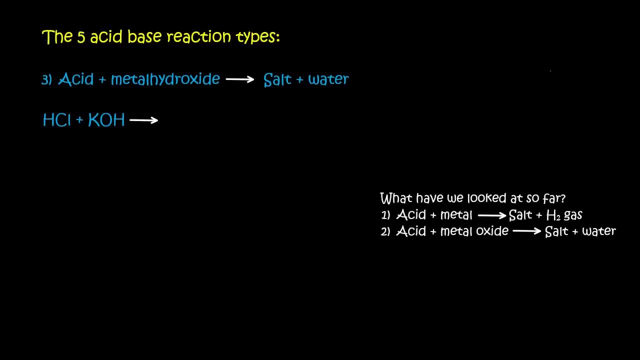 and then everything is balanced. The third one is when you have an acid plus a metal hydroxide That also gives you a salt and water, So an acid such as HCl. Now, a metal is anything from the left of the periodic table, such as potassium. 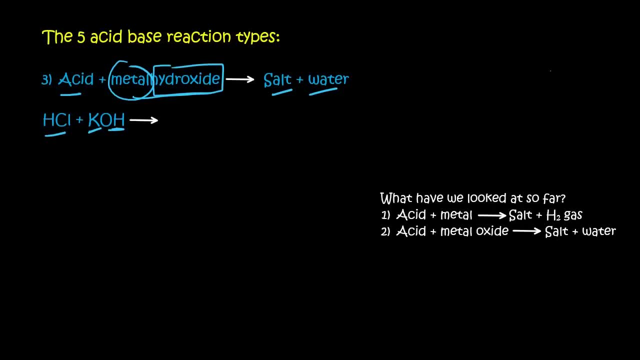 And then hydroxide is OH- Remember, it's a polyatomic iron, So it's got hydrogen and then oxygen, So it's called hydroxide. Now the product should be a salt and water, so I always put the water first And then what's left over. Well, we've got a K and we've got a Cl, so that's your salt. 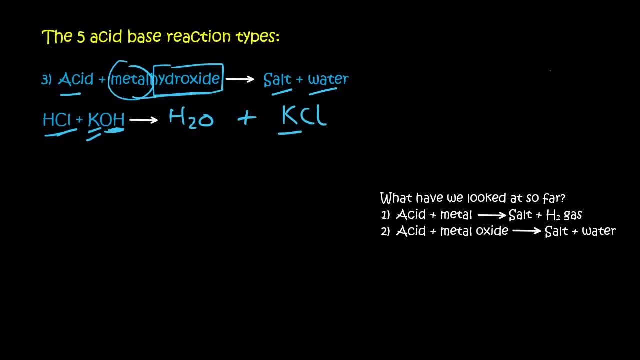 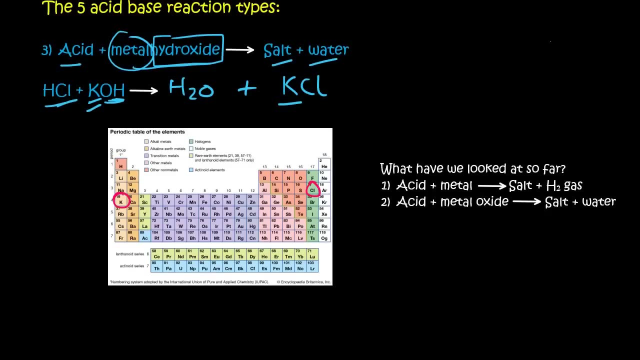 Remember, a salt is a metal and a non-metal. Now, potassium, if you look on the periodic table, has a valency of plus one and chloride has a valency of minus one, And so they are balanced already. Now we should just make sure that the reaction is balanced And if you have a look, 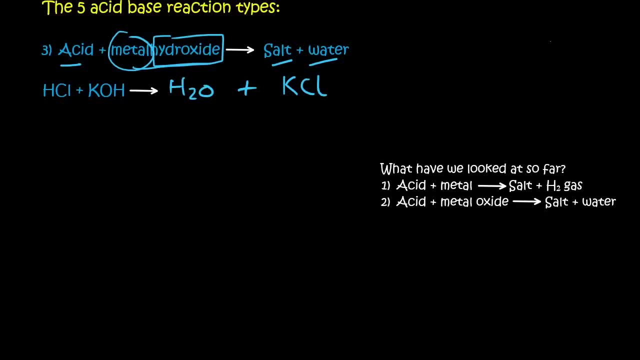 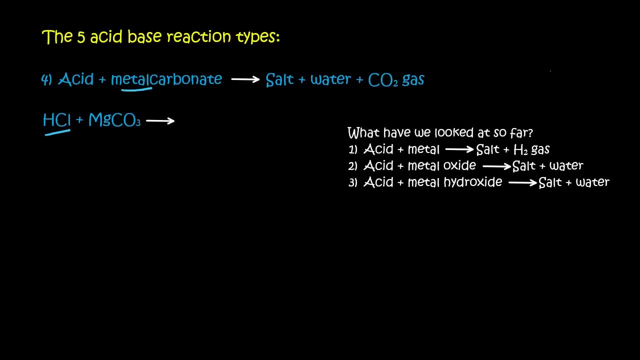 you'll see that there is the same amount of everything on each side, and so that is balanced. And so here's the fourth one. This is quite a long one. So it's an acid such as HCl, plus a metal which is like magnesium carbonate, which is CO3.. Now on your periodic table. 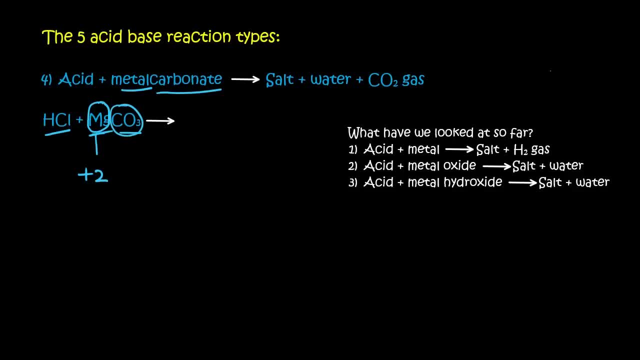 you'll see that magnesium is plus two. You need to know that magnesium is plus two. your polyatomic ions, that is minus two, And so they balance each other nicely And that is why I don't need to put a two over here. for example, Now the product should be a salt water and CO2.. 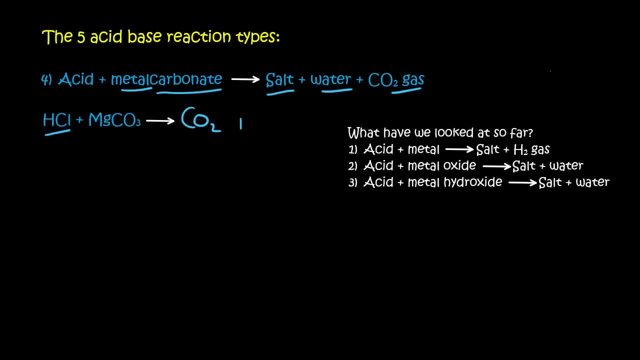 So CO2 is easy, because it's just CO2, literally, And then water is just H2O, And then, for the salt, you just see what's left over. Well, we haven't used magnesium, and we haven't used Cl, And so we 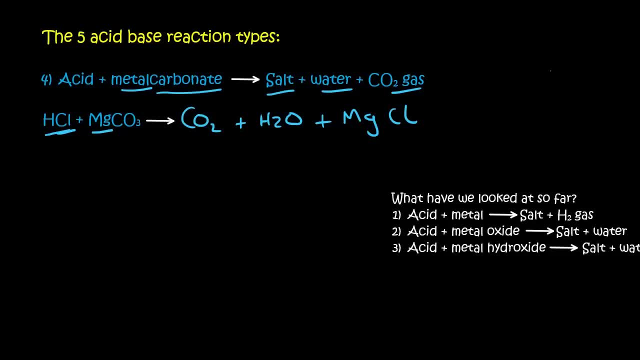 say MgCl, But now on the periodic table Mg is plus two and Cl is minus one, And so we have a two Cls And now we can balance it. So the first thing I see is that there are two Cls on this side.